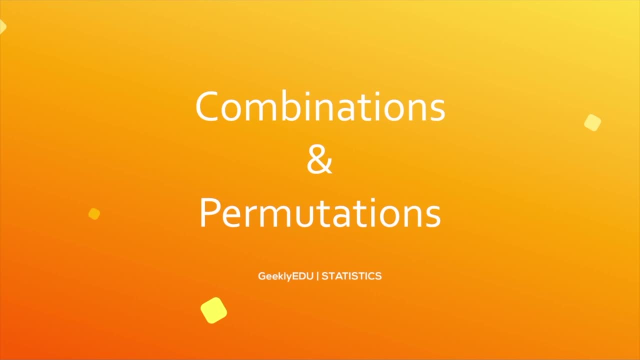 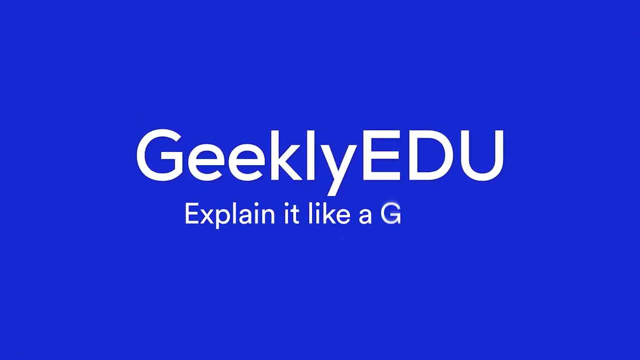 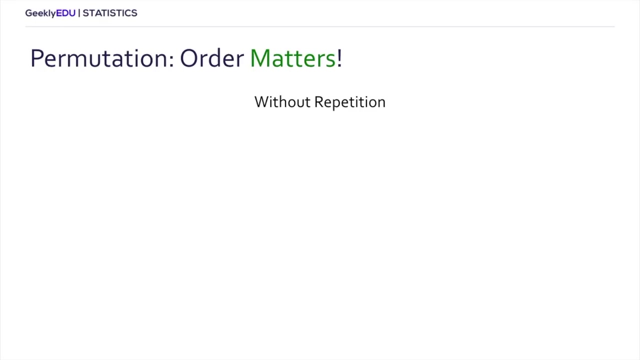 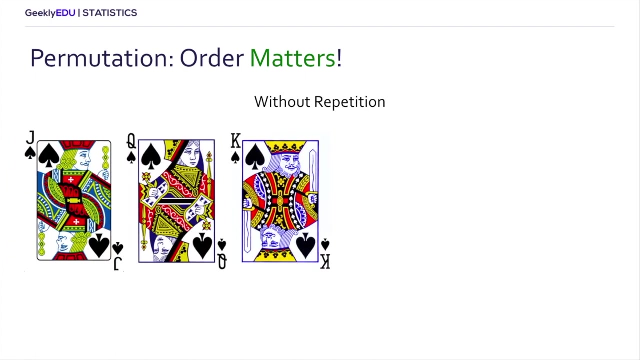 order is important and is something that we need to factor in. we'll start by talking about permutations, without repetition. here I have three cards: the Jack, the Queen and the King of Spades. now the question is: how many ways are there to arrange those cards? to answer it, we need to consider what happens every time we draw a card: the. 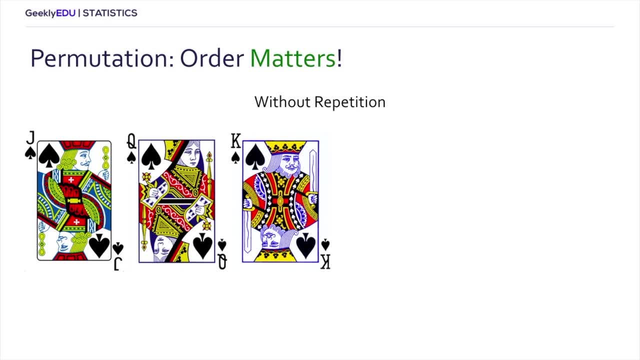 first time we have all three cards available to us. however, in the second draw we only have two cards available and only one on the last third draw. mathematically we can represent that with a factorial where we multiply 3 by 2 and by 1 and what we get is 6, so there's a total of 6 permutations that. 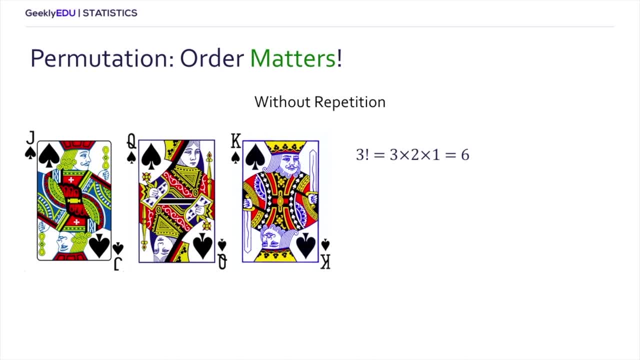 are possible with those three cards. let's consider a different question. what if we had five cards and we wanted to draw only three? now the answer is not 5 factorial, since we have only three cards that are drawn, and on the first draw we have five cards available on the second. 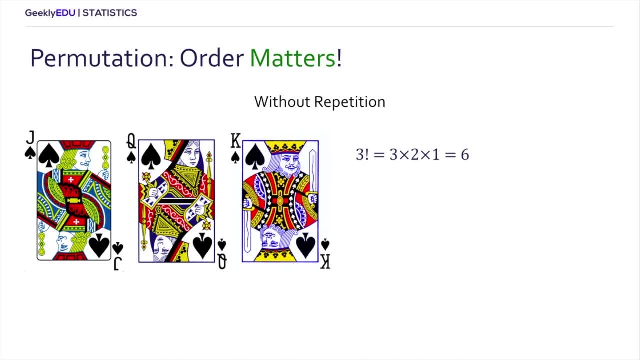 we have four and on the third we have three, so there's still two and one that we need to take care of. so to make the number accurate, we are going to put the five factorial in the denominator and we're going to put 2 multiplied by 1 or 2 factorial in the denominator, and that 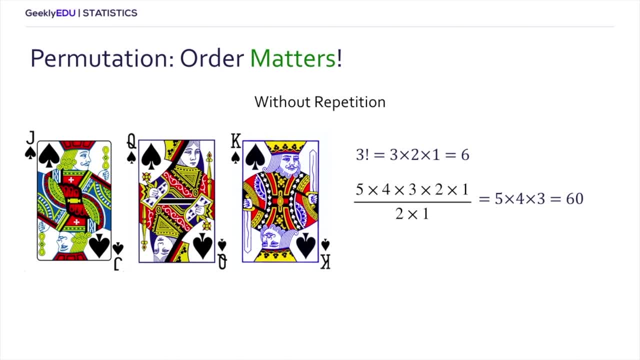 gives us the accurate answer. so we have 60 possible permutations now. the general formula looks like this: NPR equals N factorial, where N is the total number of items in the denominator in our set and r is the number of items that we are going to draw. 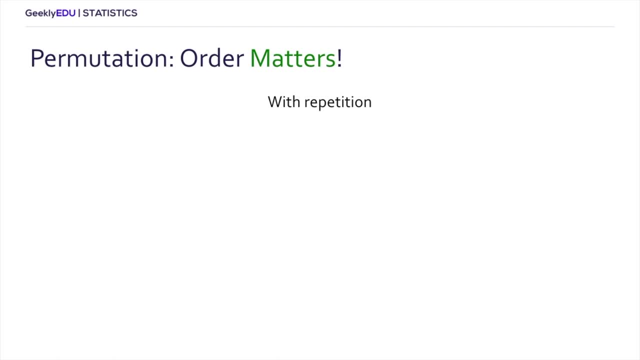 Next we have permutations with repetition. Those are a little easier than the ones without repetition and the formula is a bit more straightforward, but since we're trying to consider all possibilities, let's take a look. So here we have three balls: green, blue and yellow. 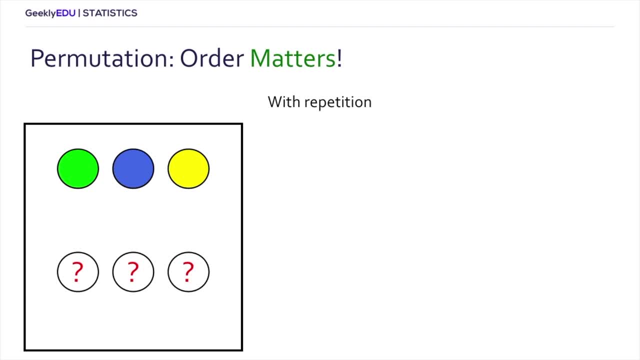 We're going to draw a random ball out of those three, three consecutive times, and the difference between the permutations without repetitions and the ones with is that in this case, whenever we draw, the range of our possibilities remains the same. so, mathematically, what that looks like is: 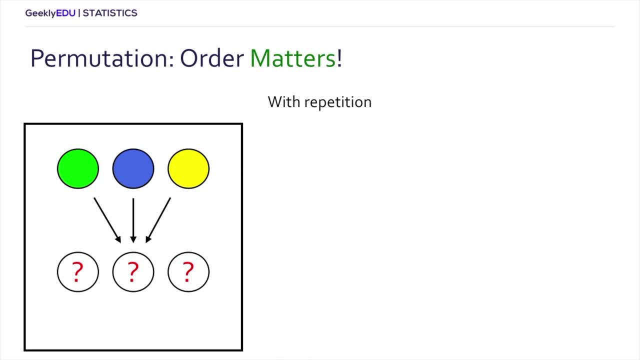 3 multiplied by 3 and multiplied by 3, or if we consider r to be the number of draws and n the number of items that we're drawing from, we can express the formula as n to the power of r, and so in our case here, n equals 3 and r equals 3, so there's a. 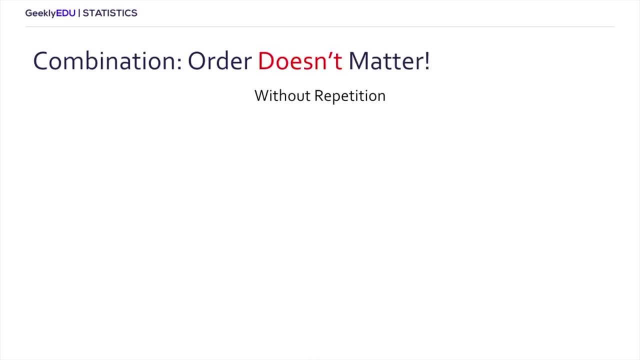 total of 9 possible permutations. Now we're going to discuss combinations, and the thing about combinations is that, unlike the permutations, the order doesn't really matter. And first we're going to look at combinations, without repetitions, since they are a little easier to wrap your head around, And 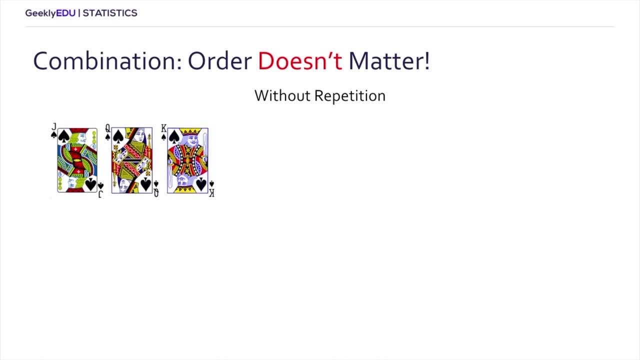 let's go back to our example with the cards. We just figured out that three cards can have six possible permutations without repetition. However, if we take a look at those permutations, there's a thing that doesn't change, it's just different. There are different arrangements of the same cards: the king, the jack and the queen, and in 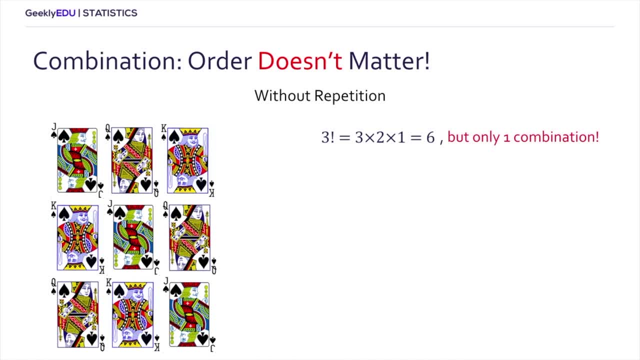 terms of combinations, there's only one. There may be six permutations, but it's still the same cards being shuffled. So let's ask a slightly different question: How many two card combinations can we draw from three cards? If we consider the possibilities, we realize that there are only 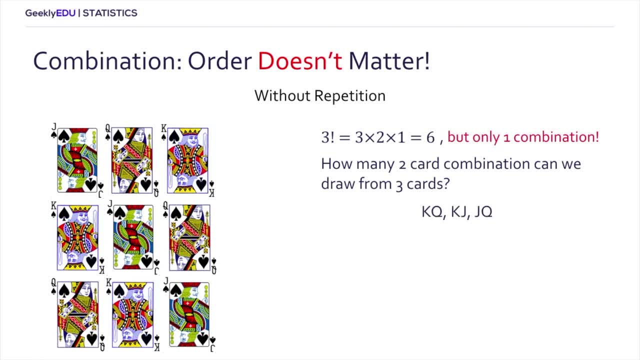 three cards. It's the king and queen, the king and the jack and jack and the queen. So, mathematically, what that is going to look like- if n is the number of items and r is the size of each combination- is this: We get this formula, which is very 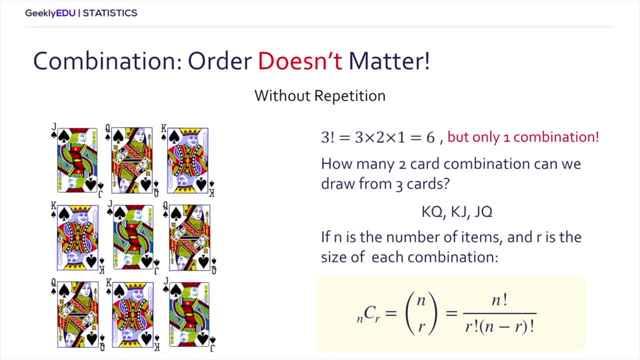 common in mathematics as well as statistics in particular, and you read it like this. the NCR is read as: n choose r Where, as I've said before, n is the number of items and r is the size of each combination, the number of items you're going to draw, and it looks well a little. 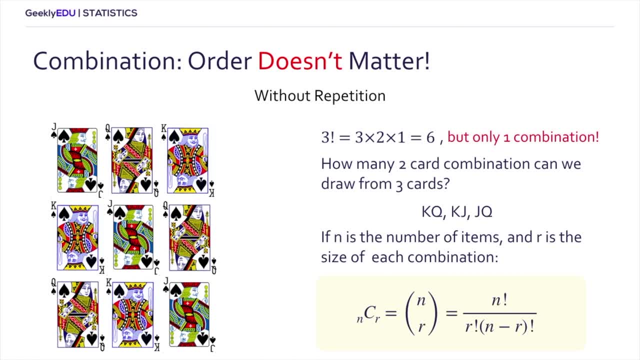 bit all too familiar, right? so it's just like the formula for permutations, without repetition. However, we are also multiplying this formula by one over r, factorial, to get rid of, you know, the repetitions. so we eliminate the queen and king, and king and queen are going to become the same thing and we 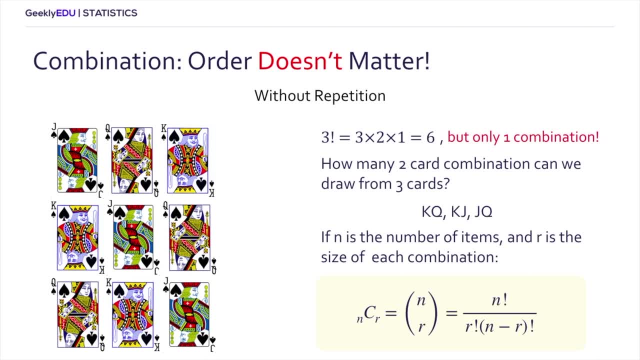 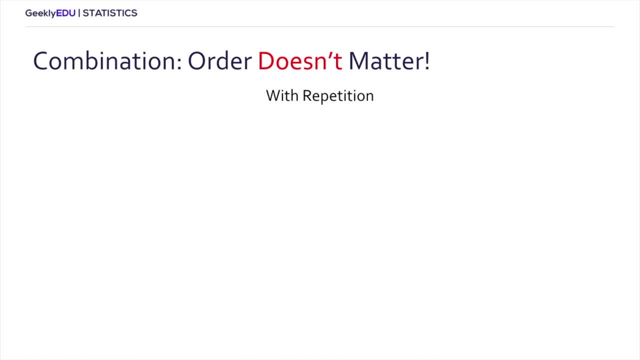 eliminate those similarities to leave only the, the combinations. Last but not least, we have to consider combinations with repetition, and I'll be honest: when it was first explained to me, it took me a while to really understand what's going on. However, once you do, it's nothing short of mathematical magic. So let's start by 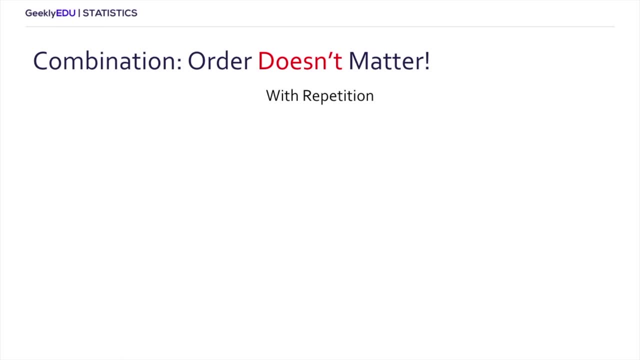 asking a question That is a variation of a different question we just discussed: How many two card combinations can we draw from three cards? However, this time with repetition, To answer that, we'll start by drawing a table. Here we have a table with three columns where each column represents a. 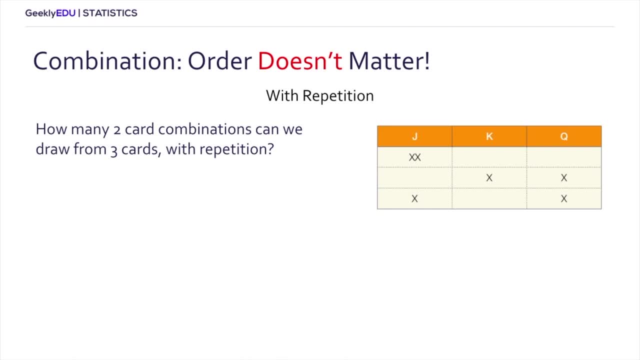 type of card- The Jack, the King and the Queen- that we've seen before, and each row represents a particular combination. So in the first row we have two Jacks. in the second row we have a King and a Queen and a Jack and a Queen. 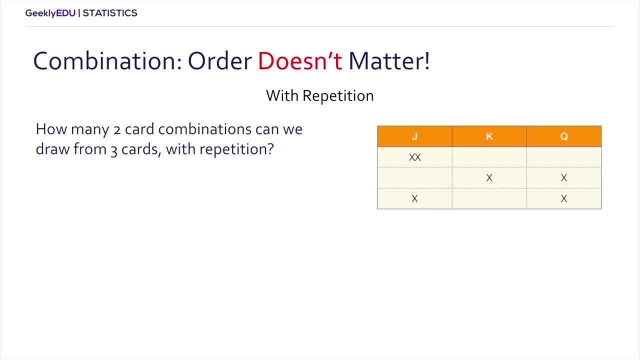 in the third row. If you look at this table, you can actually see that there's a way to simplify and make it more abstract, and it's going to look something like this: See, in this kind of coded language, we can express into which bin or which column. 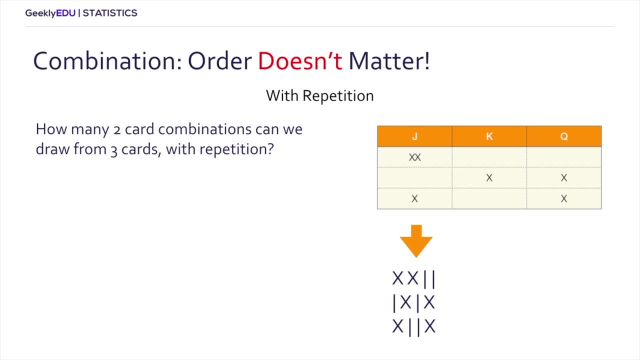 every particular item we draw goes, and by arranging those X's and those lines in a particular fashion, we can figure out how many items of a particular category we have and thus determine what combination this is. So, if you're starting to realize where this is going, brilliant, because this is the part that 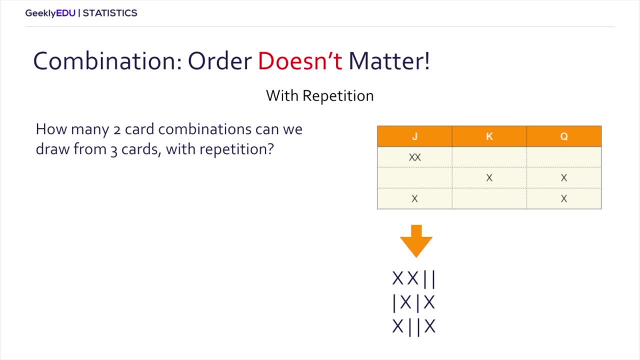 took me a long while to wrap my head around, and what we do next is we put those axes and those lines in their own distinct cells. It helped me to number them to really see what's going on and what you have. those numbers are actually their own set, from which we can. 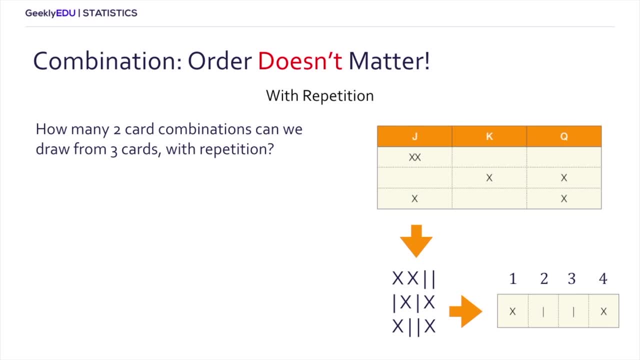 draw, and that means we can make combinations with it, right? So, for example, what you see here is a combination of 1 & 4, if you took the axis, or if you took the lines as a combination of 2 & 3.. So we start to see. 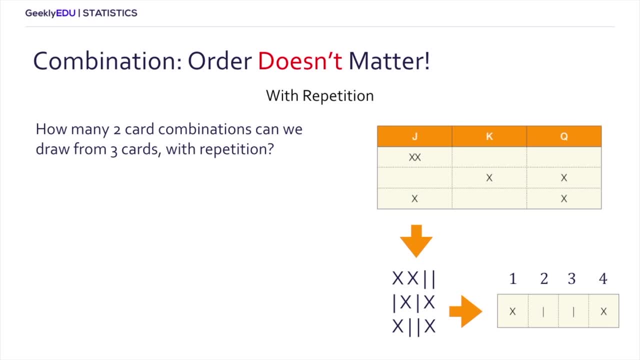 that every particular combination here corresponds to a particular combination in our original problem. So X line. line X would mean that there's one jack, no king and one queen. In essence, we just took a complicated question and asked a slightly simpler. 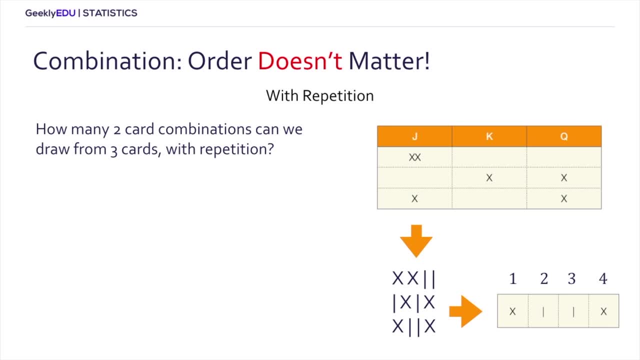 one, one that we know how to answer, And the question is: how many ways are there to arrange the axis and the lines in those four cells? And yep, you got it right. this is a question about combinations without repetition, since every cell has its particular number assigned to it. 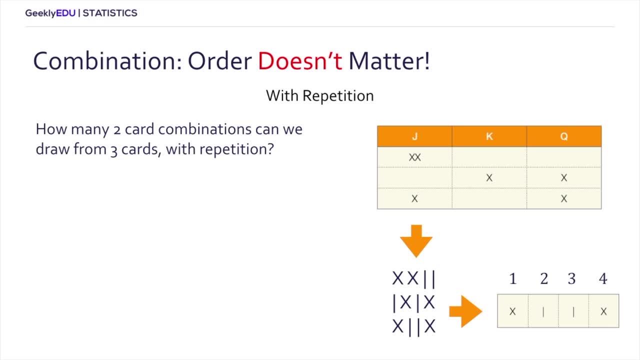 So the mathematical answer to it looks like this: it's 4 choose 2. that equals to 4 factorial divided by 2 factorial and 4 minus 2 factorial, which gives you 24 over 4, or a total of six possible combinations. And the six combinations of X's in those four cells is actually the. 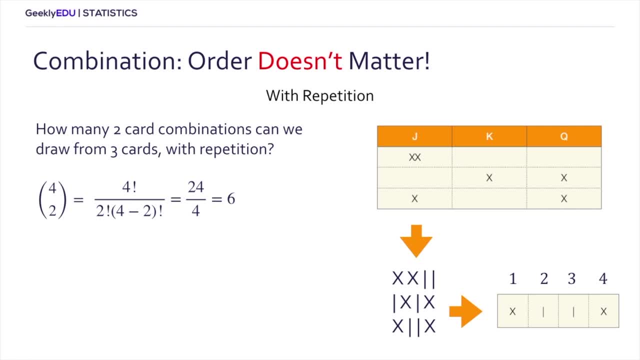 six possible combinations of cards that you can have if you draw two from a stack of three. Let that sink in. The question wasn't answered directly. rather, we took a sidetrack to simplify what we were asked and then give a direct answer to the problem through an indirect.